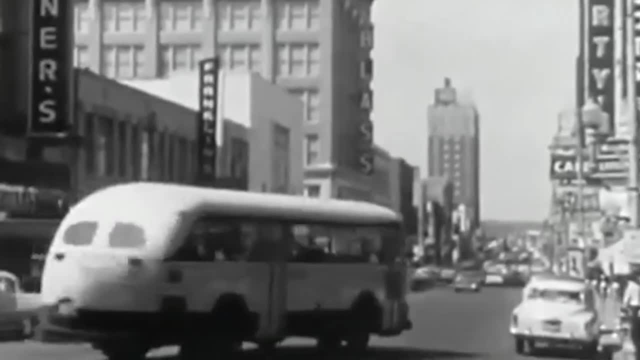 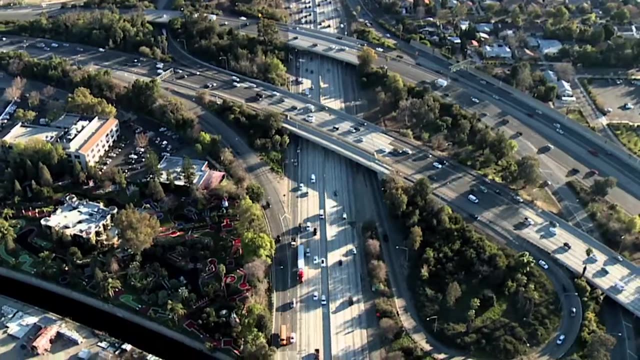 It might be a little different than you think. Before, about 1960,, most cars used generators to drive the electrical system and gas to run the engine. Most modern cars use an alternator, which is a slightly different kind of generator for the electrical system. 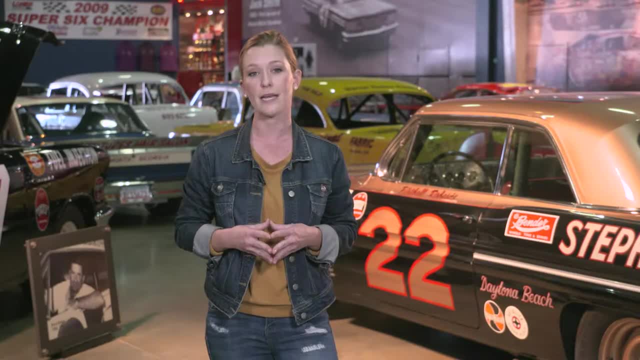 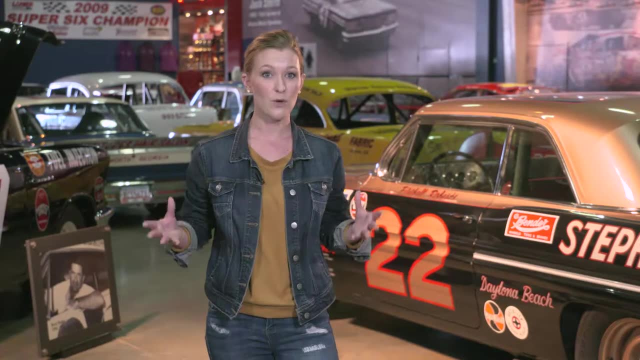 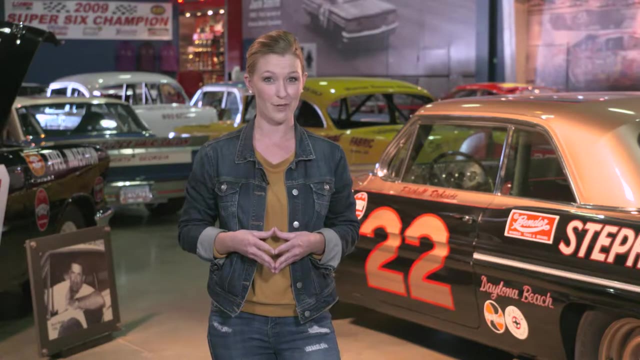 But motors and generators both use electromagnetic induction, in which voltage is induced by a changing magnetic field. Okay, so you know that electricity can generate a magnetic field and vice versa, But what you may not know is that this discovery, hundreds of years ago, led to figuring out 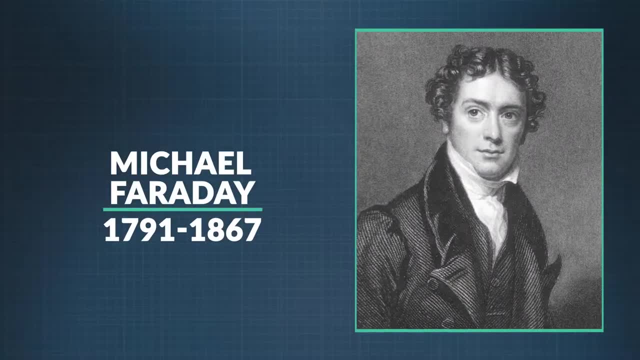 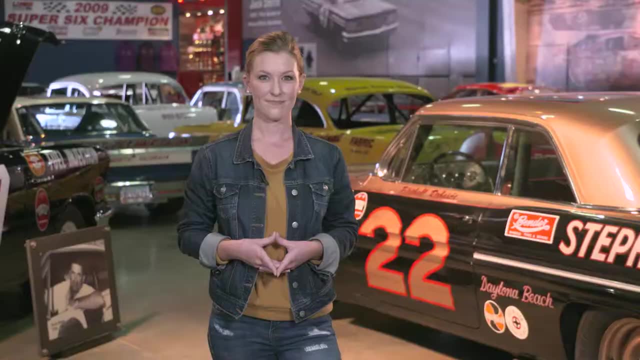 how to build a car, and it starts with a man named Michael Faraday. He's the guy who invented the generator, which changed just about everything having to do with how they work. Today he's considered one of the greatest scientists who ever lived. 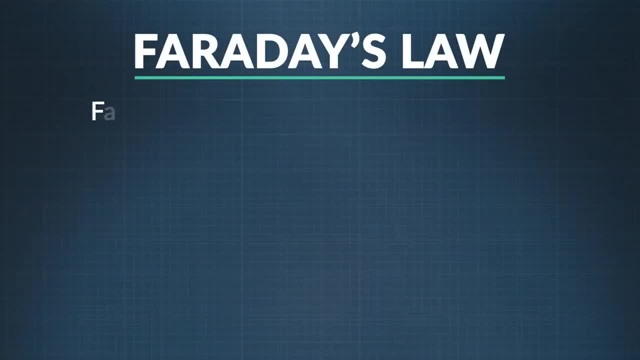 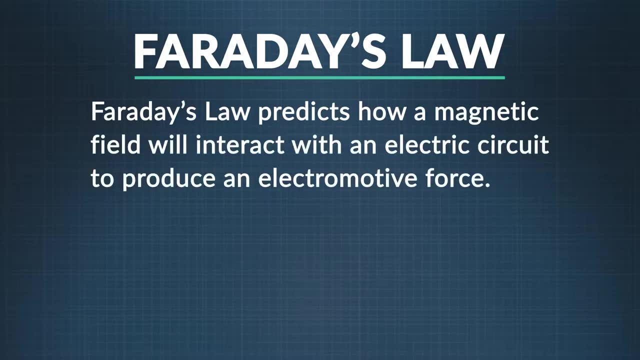 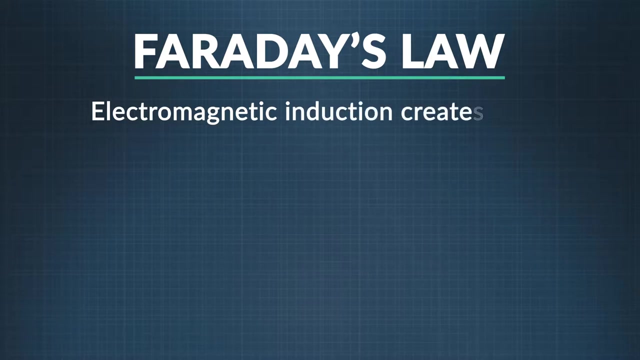 One of his many legacies is called Faraday's Law. It predicts how a magnetic field will interact with an electric circuit to produce an electromotive force, or EMF. This interaction results in the phenomenon we call electromagnetic induction, which creates a current in a circuit when there is relative motion between the wire and the magnetic field. 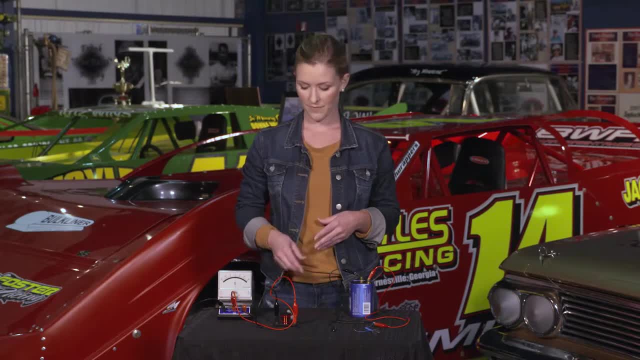 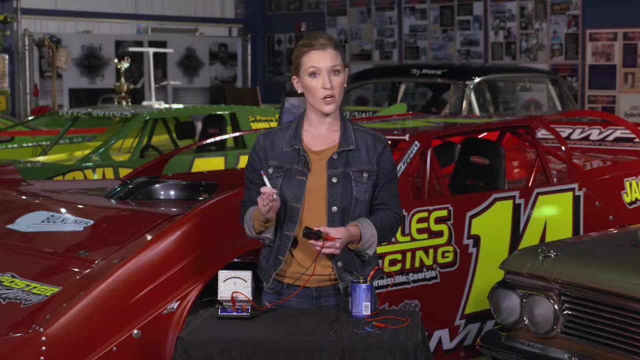 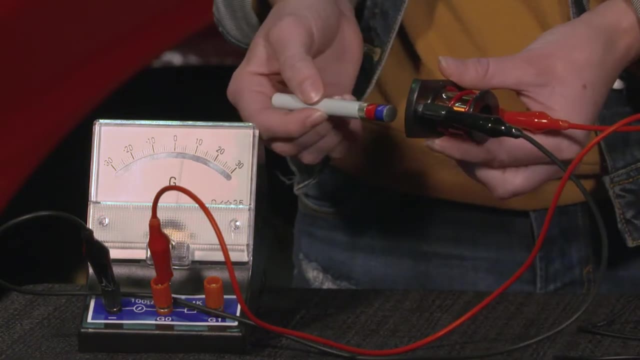 I'll show you how it works. Here's how it works. I'll show you in a simple demo. When I put this magnet through this wire loop, the changing magnetic field creates a current in the wire. You can see it here on the voltmeter. 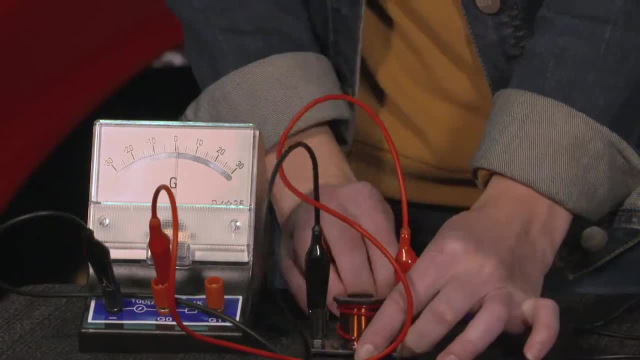 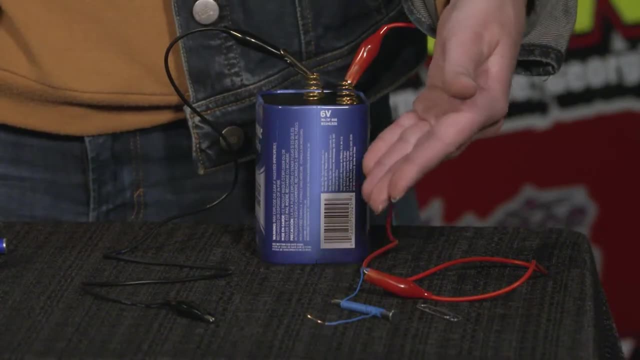 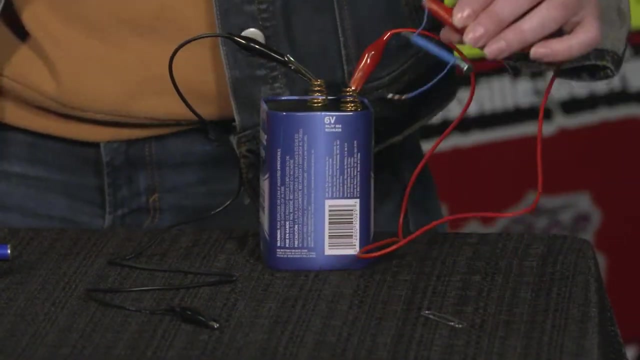 It induces a voltage and that difference in potential causes current to flow. You can also see how electric current induces magnetism with this wire, nail and battery. This nail is not a magnet, But when it's wrapped in a coil of wire and I cause the current to flow by attaching it. 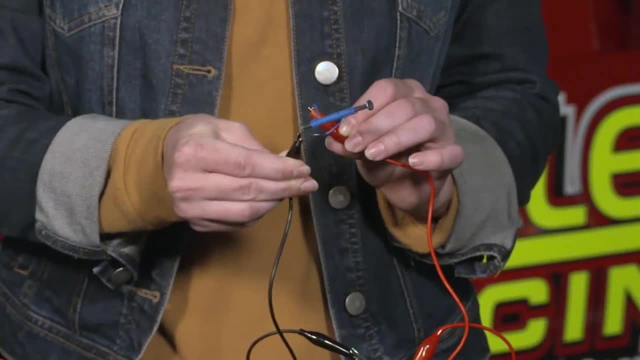 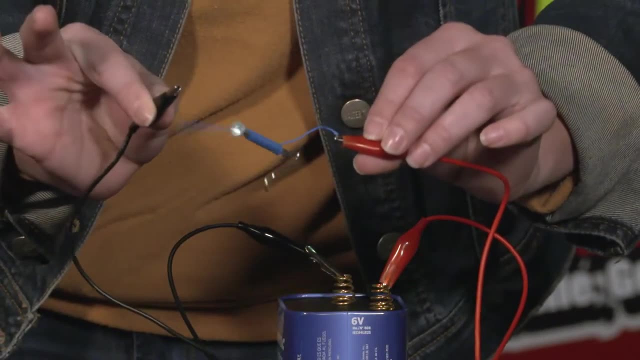 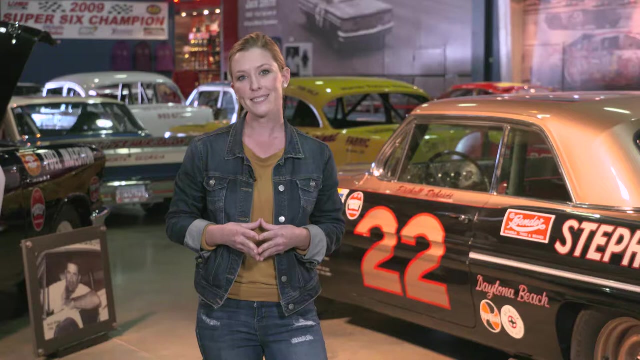 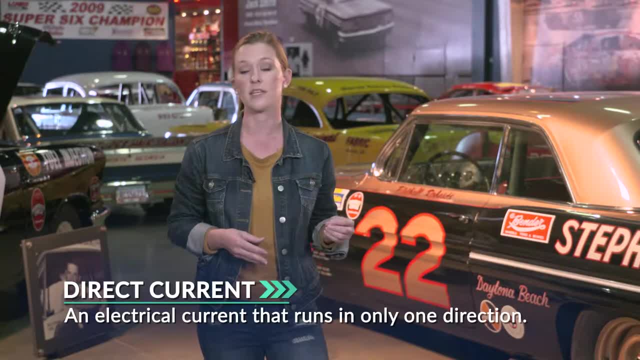 The most basic type of motor is a DC or direct current. The most basic type of motor is a DC or direct current. Direct current is electrical current that runs in only one direction. Current travels from a battery and moves through wires called brushes. 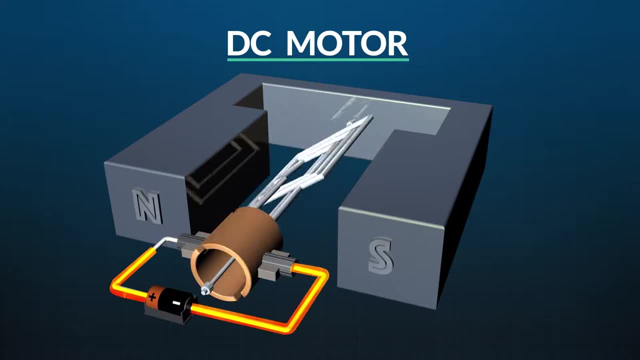 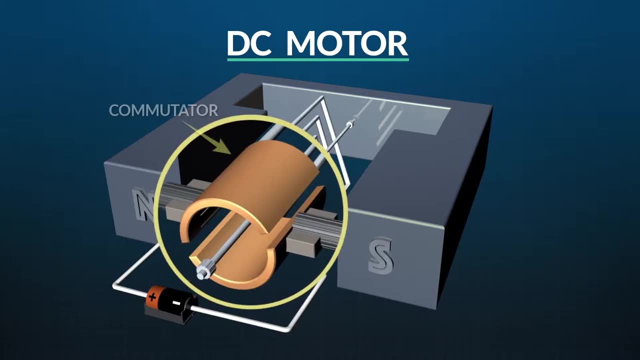 because in the old days they actually were brushes. Today there are also brushless motors which use digital sensors to perform the same task. The brushes sit on a piece of metal called a commutator. The commutator is a split ring, usually made of copper, that is connected. 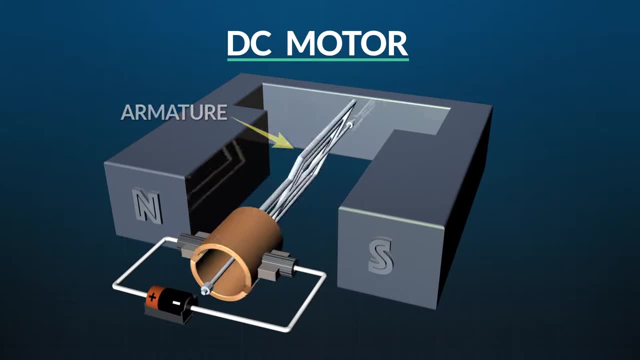 to wire loops, known as the armature. The commutator armature assembly is known as the rotor, which rotates at the center of the motor. The brushes or sensors are connected to the battery and make contact with the commutator. 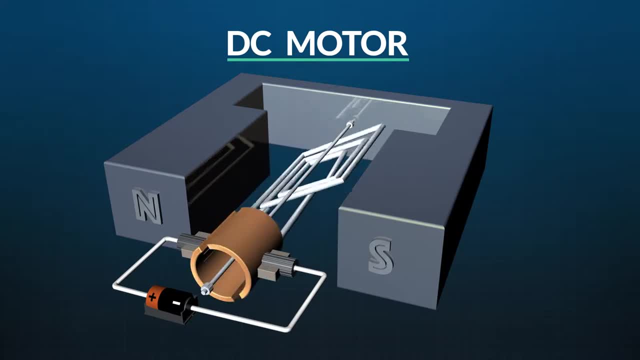 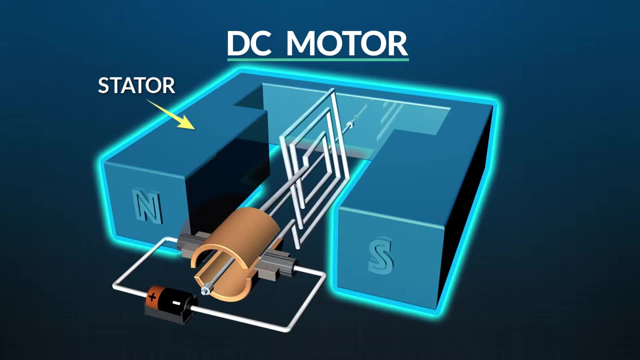 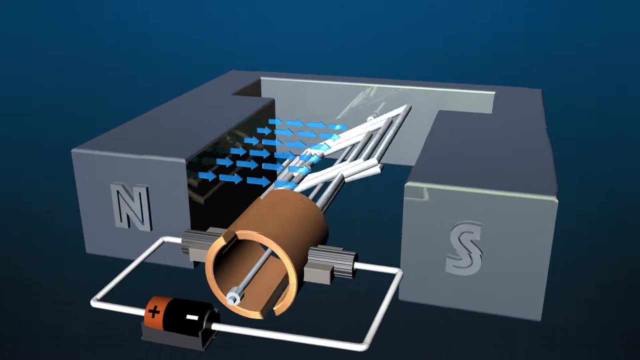 as it turns, supplying it and the armature with current. This assembly sits in a stationary magnetic field that is created by the stator, made of either a permanent magnet or coil-wrapped metal plates that surround the stator. The field exerts a magnetic force on the wires, which causes the rotor to turn. 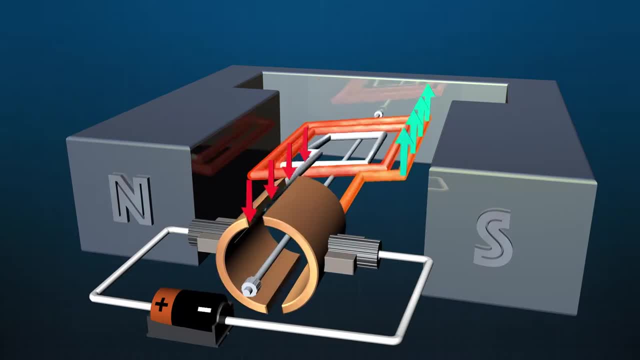 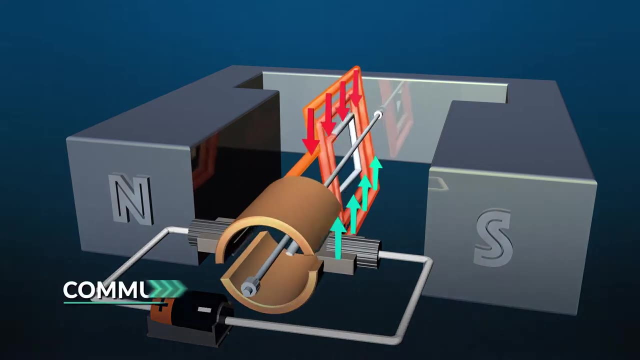 When the rotor has made half a turn, the current begins to flow in the opposite direction, because the commutator is now touching the opposite side of the battery. This electromechanical process, by which direct current is turned into alternating current, is known as commutation. 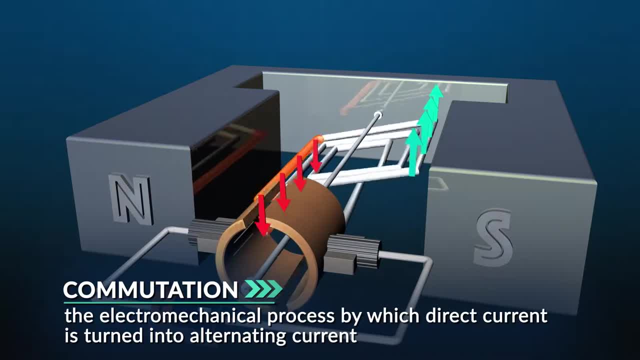 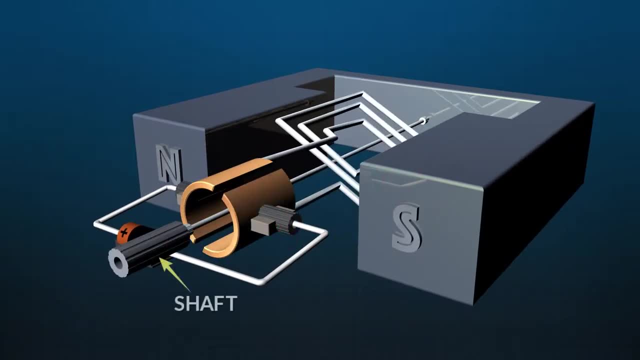 That reversal of current causes the magnetic force to shift, acting on the rotor to reverse direction. when it reverses it makes the rotor spin. that motion, that mechanical energy can turn a shaft, which is connected to many things to make them run. your house probably has at least 50 motors in it. 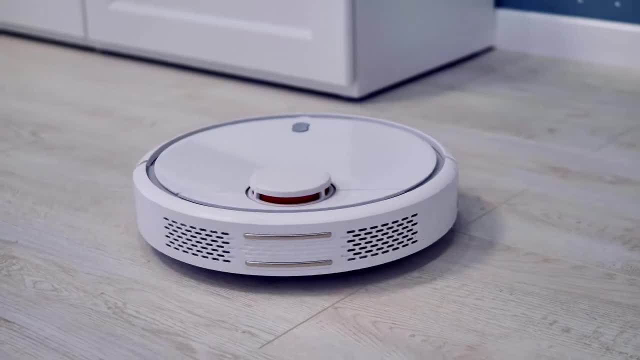 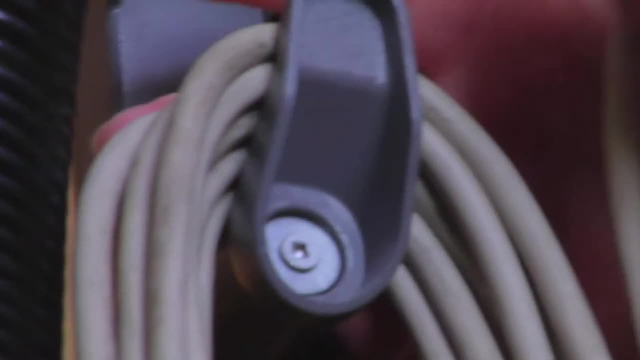 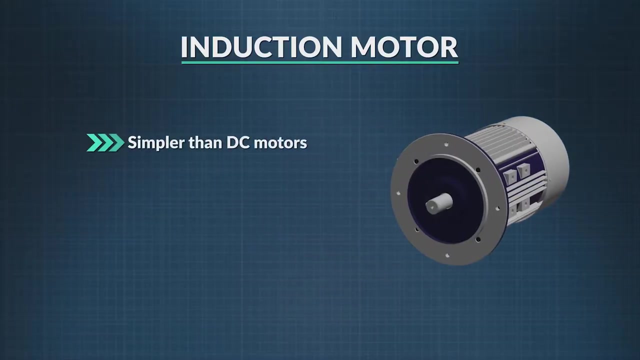 running everything from power tools and fans to household appliances and electric cars. there's another type of motor, an induction motor that runs directly off alternating current. compared to DC motors, induction motors are simpler and have fewer parts, no brushes and no commutator, which makes them more reliable and longer-lasting. while induction motors run on, 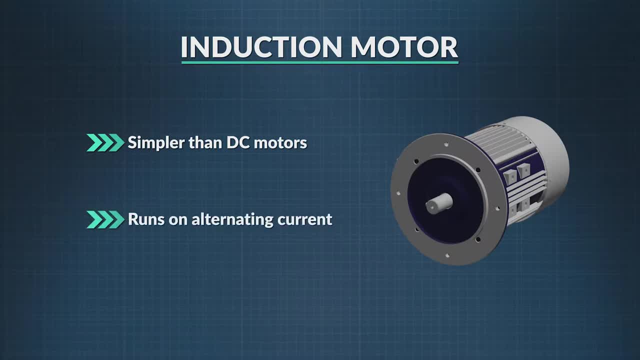 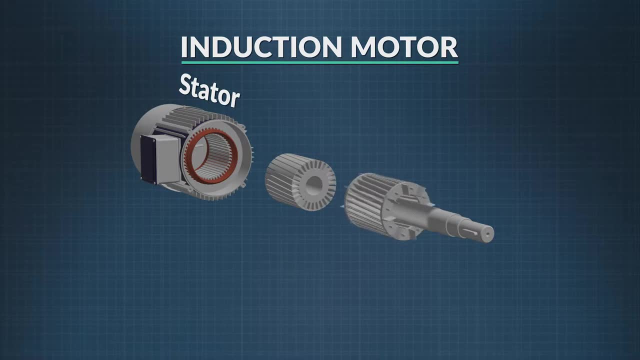 alternating current DC motors run off direct current and are used whenever the motor is battery operated. this is the stator, which in this kind of motor, is made of laminated magnetic metal plates. it doesn't move, it's stationary, just like in the DC motor copper or other. 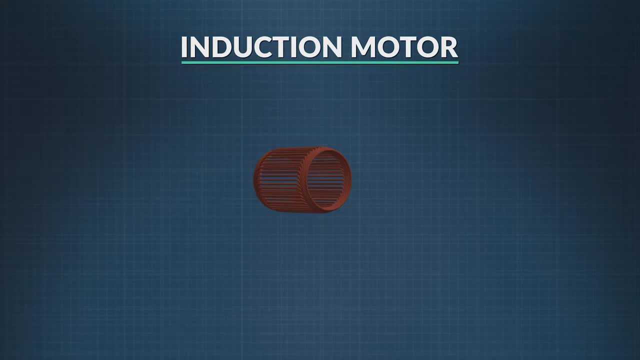 metal is wound through to form a coil. sometimes we call them windings. the more loops the windings have, the greater the magnetic field is through them. when you hook up the alternating current to the stator, the changing nature of the current flow creates a rotating magnetic. 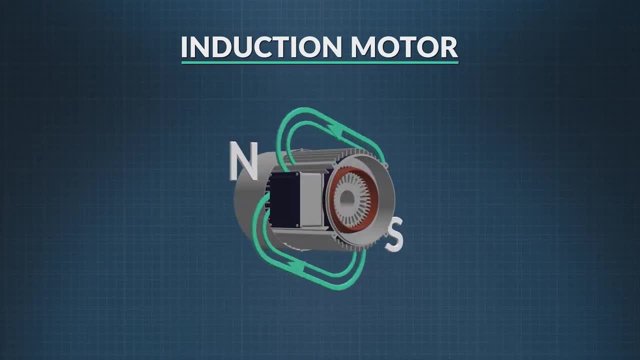 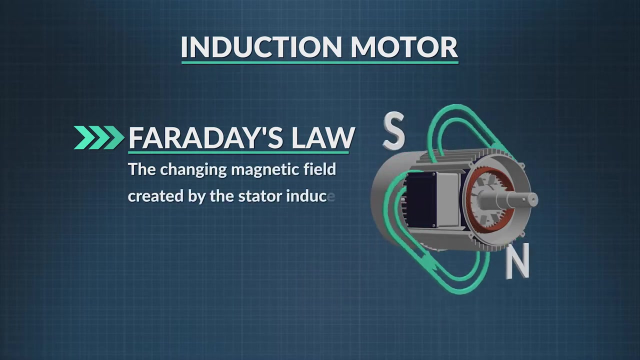 field around it. the stator doesn't move, just the field around it. like DC motor, induction motors have a rotor at the center made of copper wires. remember Faraday's law tells us that the changing magnetic field created by the stator induces voltage in the rotor and because of that induced voltage, the rotor 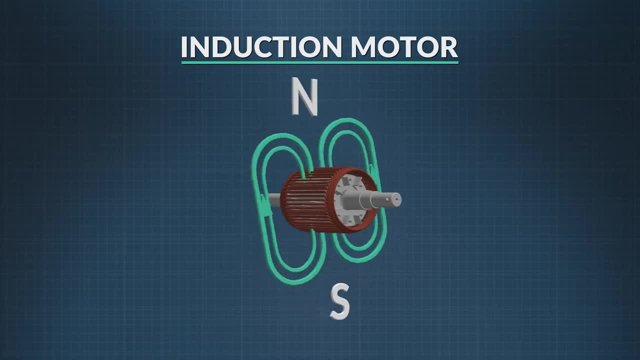 located at the center of the motor becomes a current carrying loop. the changing magnetic field around the stator exerts a magnetic force on the current carrying rotor which causes it to rotate. as the magnetic field moves around the rotor, it exerts a force in just the 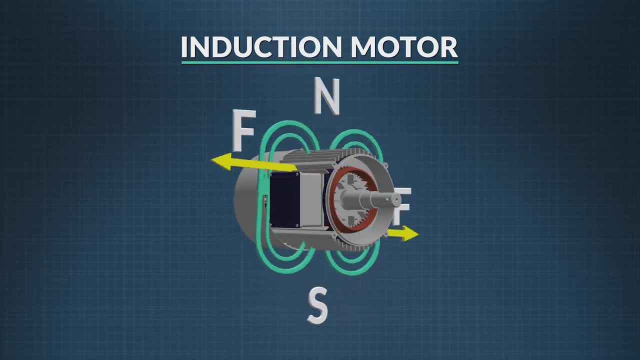 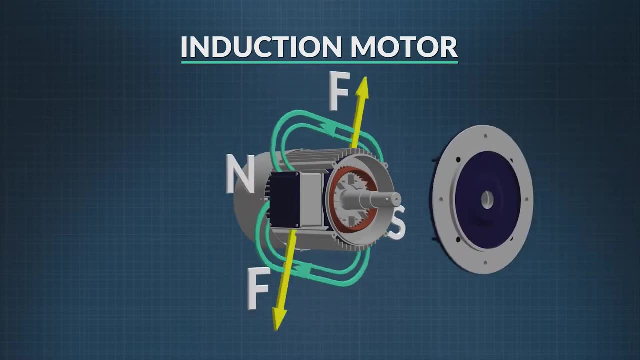 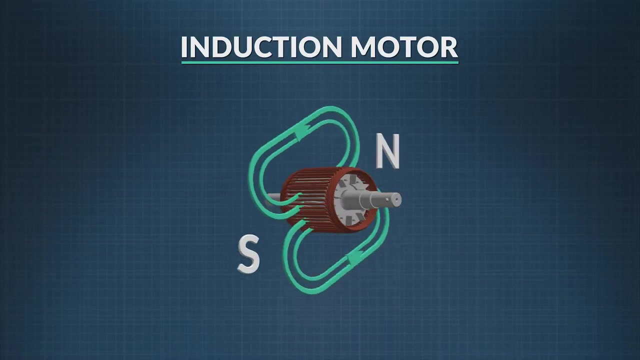 right place to cause the rotor to continue to rotate. that's what causes the rotor to spin continually, exerting a force on the wires at just the right time to create optimal power. we've seen that electricity and magnetism are intrinsically related: alternating current flowing through the wire in the 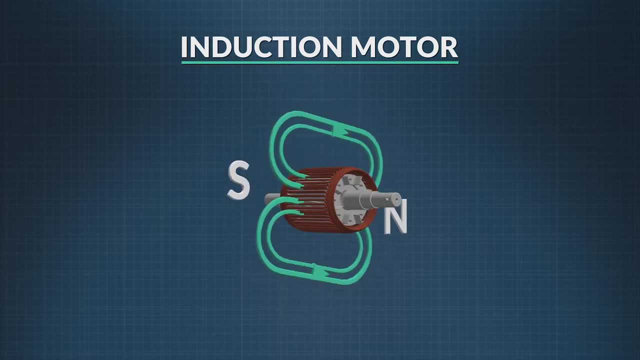 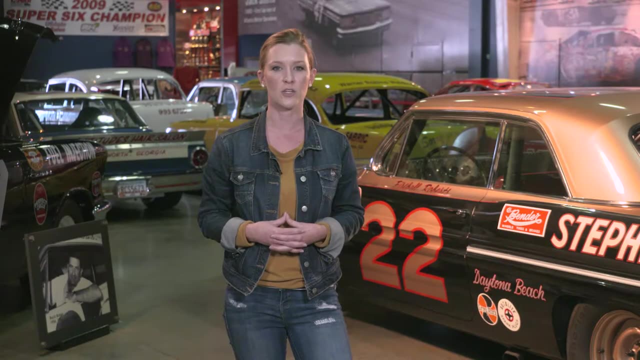 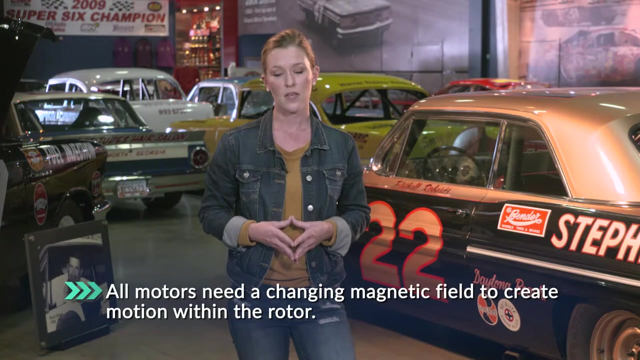 stator creates a changing magnetic field and, conversely, current flows in the wires of the rotor. because of this magnetic field, all motors function in much the same way and that they all need changing magnetic fields to create motion within the rotor. the fundamental difference between induction and DC. 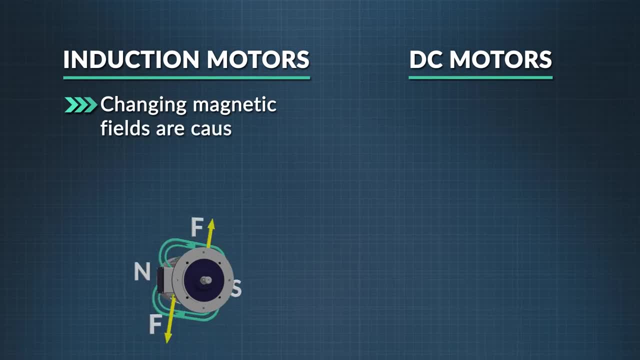 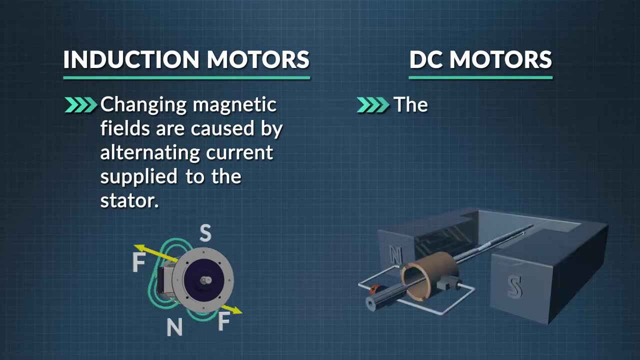 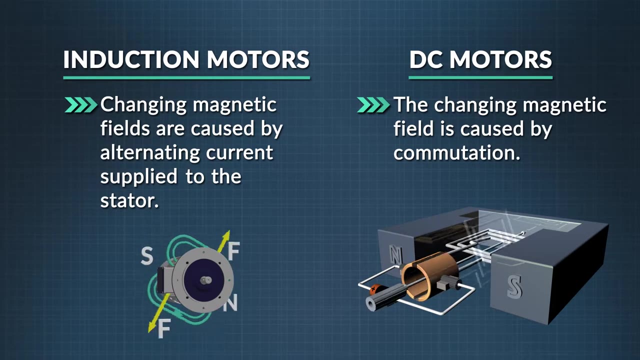 motors is that the changing magnetic fields in an induction motor are caused by the alternating current that is supplied to the stator. in a DC motor, the changing magnetic field is caused by commutation, which, as you recall, is a mechanical transformation of the direct current from the battery to 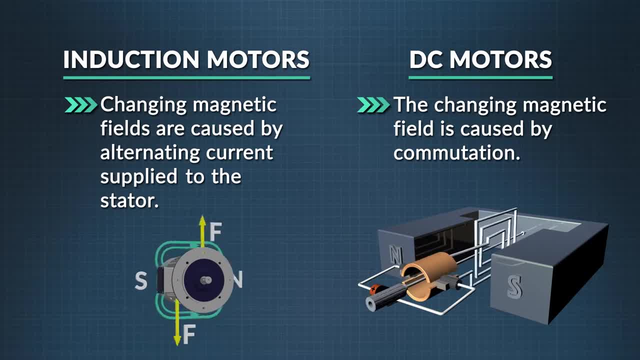 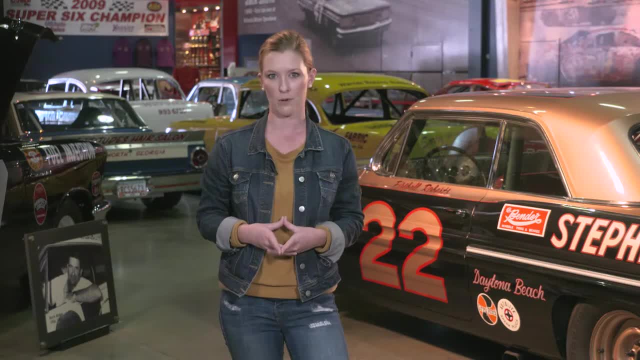 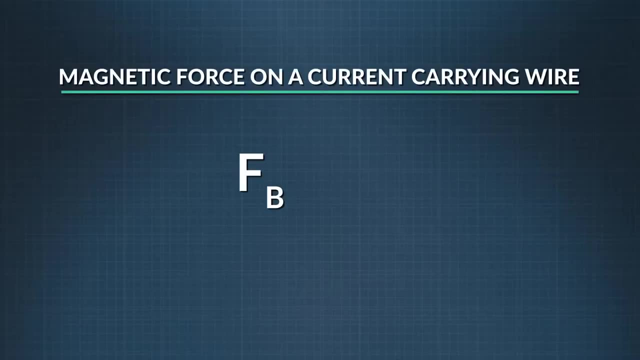 alternating current through the brushes and commutator bars on the armature that make up the rotor. let's step back a second and think how we could make this motor even more powerful. let's use the equation that allows us to find the magnetic force exerted on a current carrying wire. where magnetic force 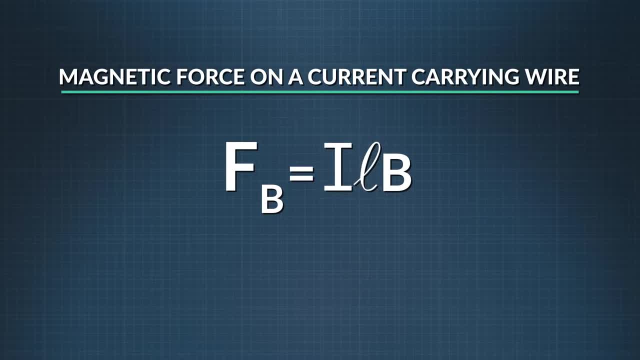 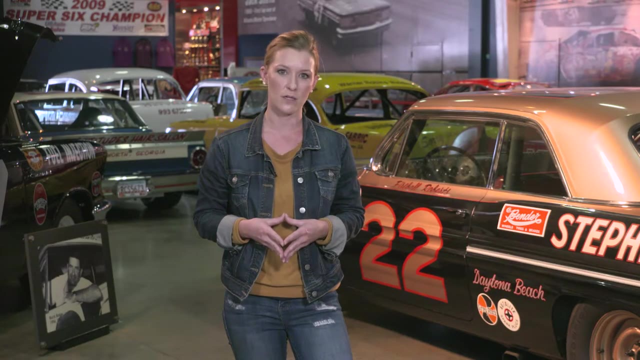 equals current times the length of the wire times the magnetic field strength. we can. we could make the magnetic field stronger, or we could increase the length of the wire, or we could add more charge and increase current. of all these options, the easiest one is to increase the length of the wire. we do this by 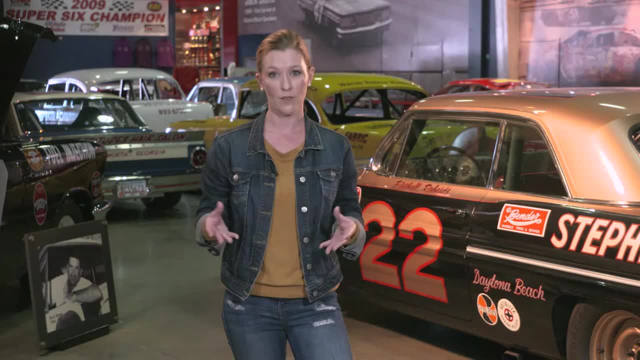 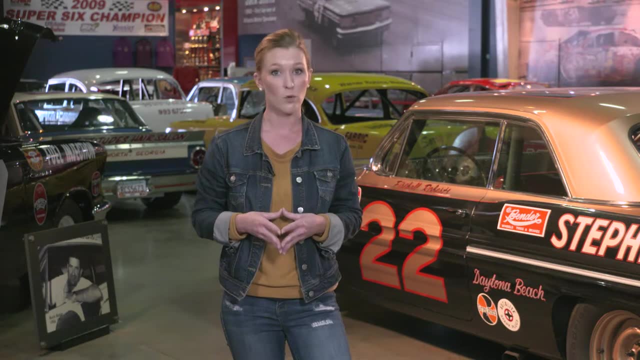 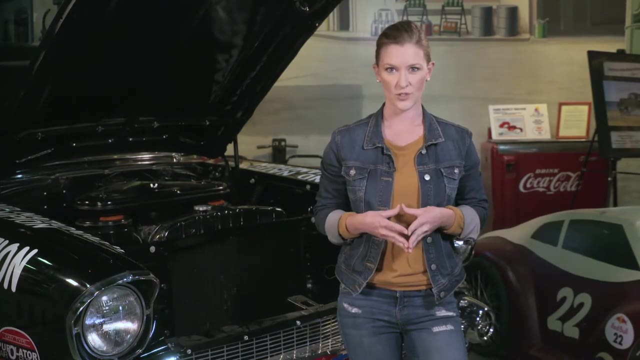 stacking loops of wire on top of each other and the coil that we've talked about. each loop contains moving charge that experiences a magnetic force. the more loops, the stronger the net force of the rotor and so the more powerful the motor. now that we've seen how motors work, let's take a look at how generators. 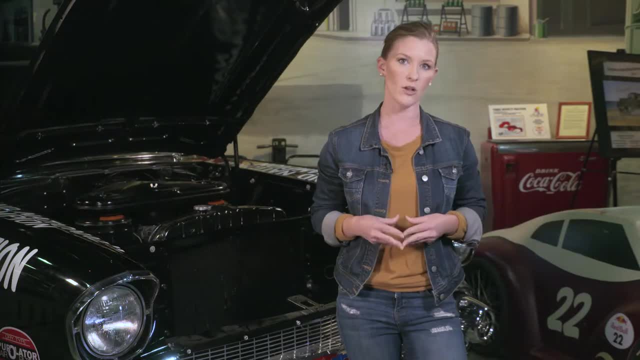 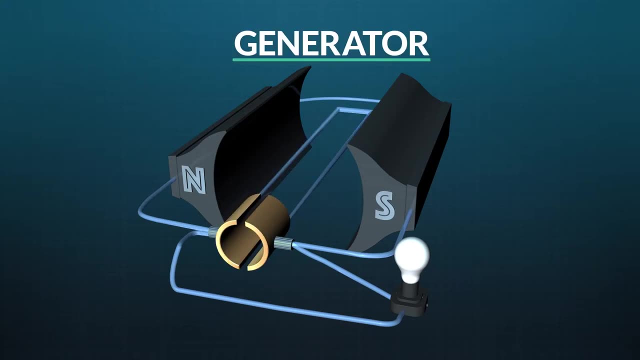 work opposite the way motors do. they take mechanical energy and turn it into electrical energy. this is a generator. it's found in classic cars built before 1964. just like certain types of motors, it has a rotor made of an armature and a commutator that are in contact with brushes, and an electromagnetic stator that 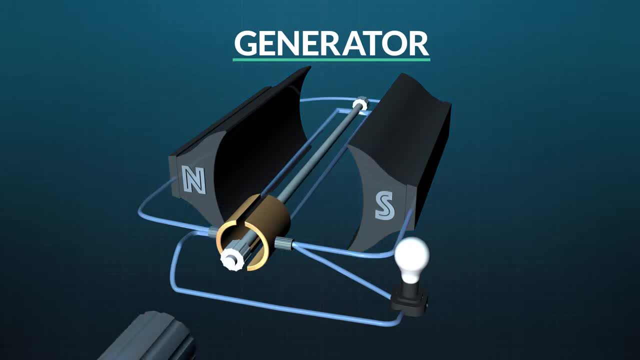 surrounds the rotor. the difference is the armature rotates through mechanical action provided by the engine being linked to it through a pulley. there's a residual magnetic field within the stator that provides the initial push to start current flowing through the armature as it rotates, some of the 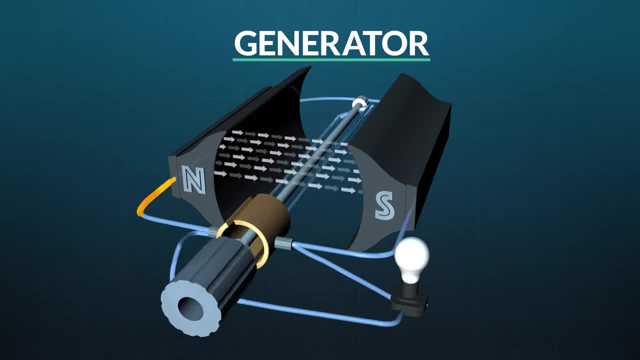 current produced by the moving armature flows to the stator, strengthening the magnetic field and increasing output in this car. the excess current from the armature is used to power things like headlights and turn signals, as well as charge the car's battery. there are many different kinds of generators, but they all follow. 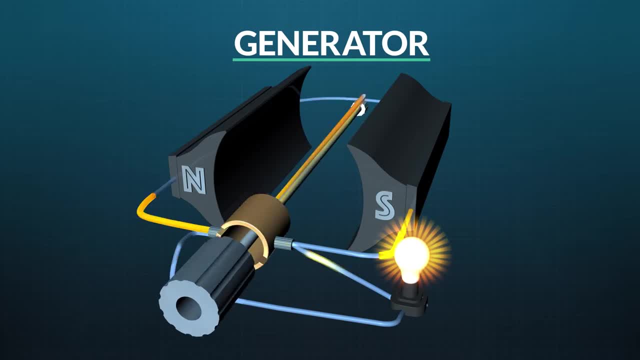 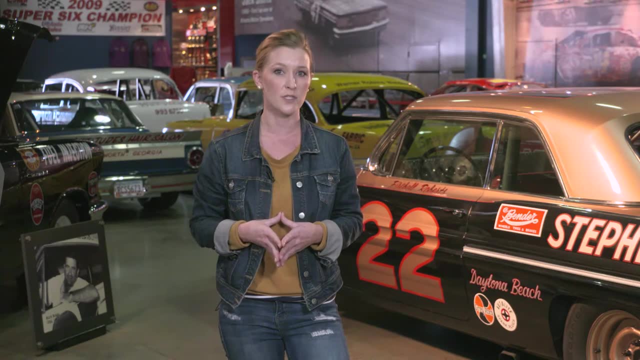 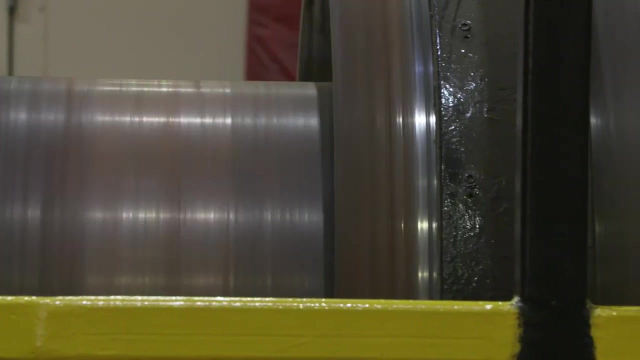 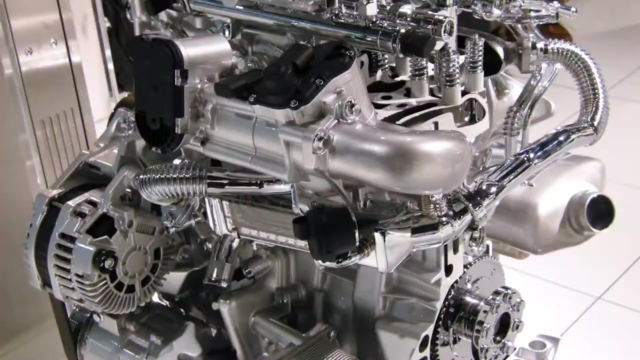 the same principle, taking mechanical energy and turning it into electrical energy. so question: between motors and generators, which one do you think supplies electricity to your home? that would be a generator. so a power plant consists of an electrical generator. something has to spin the rotor within that generator. It might be a water wheel in a hydroelectric dam, a large diesel.